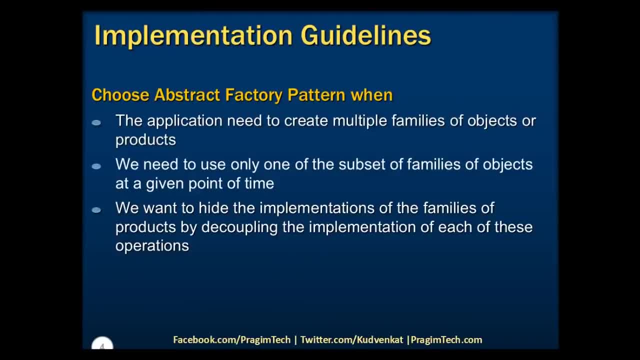 Now let's take a look at the implementation guidelines of abstract factory. We need to choose abstract factory pattern When the application need to create multiple families of objects or products And when we need to use only one of the subset of families of objects at a given point of time. 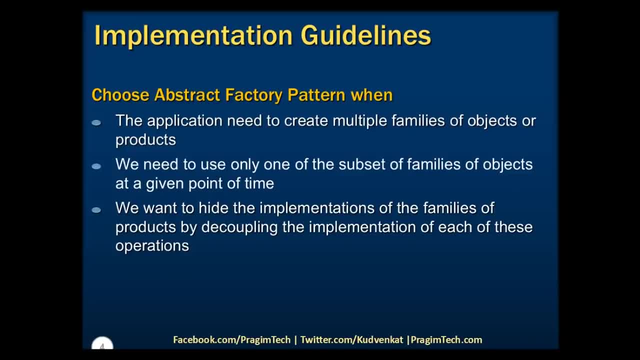 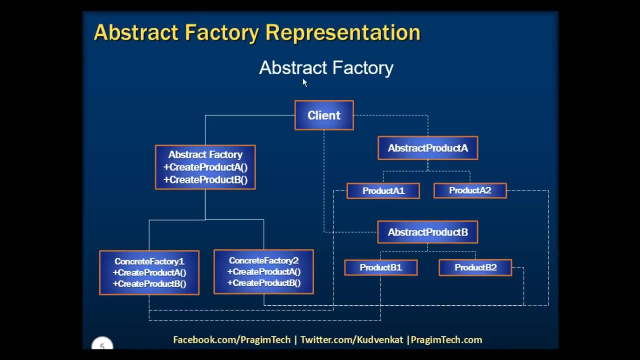 And when we want to hide the implementation of the families of products by decoupling the implementation of each of these operations. Now, if you take a look at the illustrated diagram of abstract factory representation, The client is a class which uses abstract factory And abstract product interfaces to create a family of related objects. 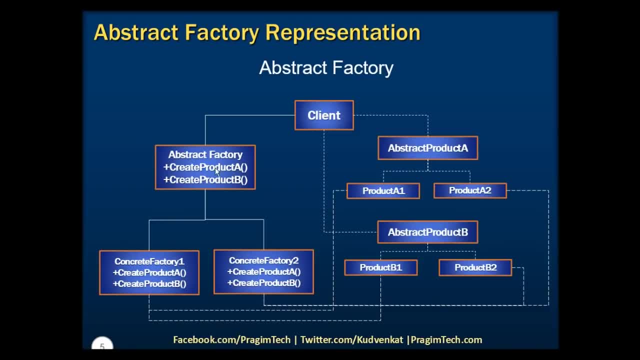 Abstract factory is an interface which is used to create abstract product. Concrete factory is a class which implements the abstract factory interface to create concrete products. Abstract product is an interface which declares a type of product. Concrete product is a class which implements the abstract product. 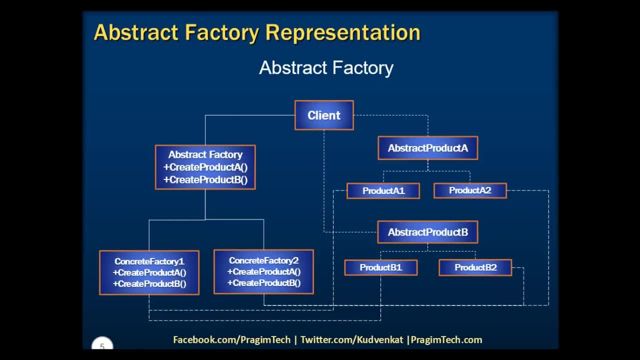 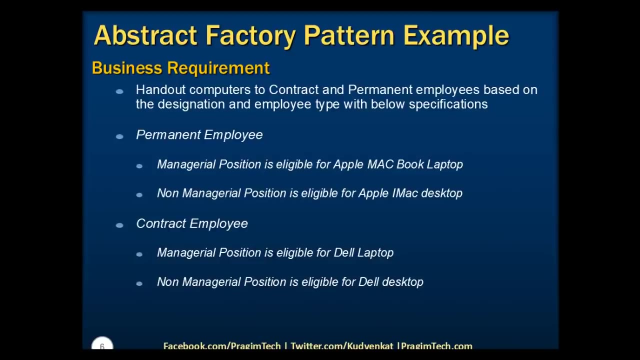 interface to create product. If this is confusing at this moment, don't worry, as we are going to take a deep dive on implementing these points using a simple example. Now let's consider a business requirement where a company decides to hand out computers to contract and permanent employees based on the 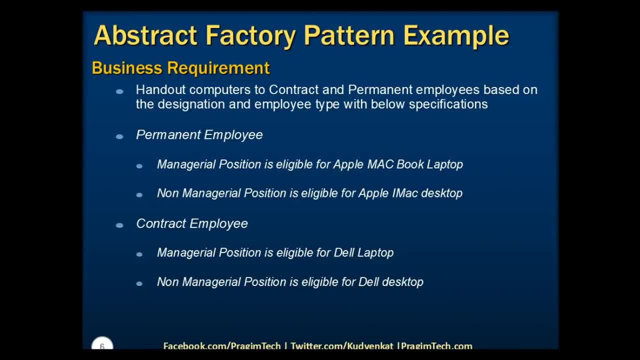 designation and employee type with below specification. Let's say, a permanent employee who is a manager is eligible for Apple laptop and rest of non-managers are eligible for Apple desktop, Whereas in case of contract employee who is a manager is eligible for Dell laptop and rest of non-managers are eligible for. 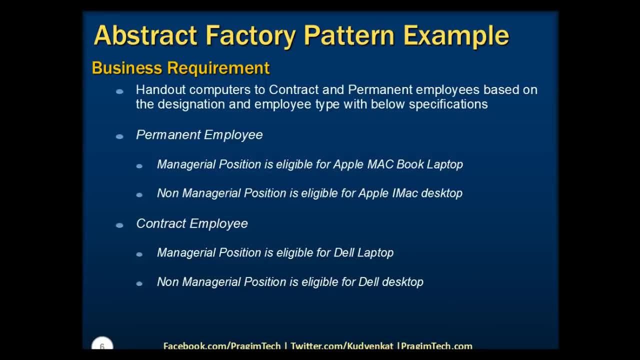 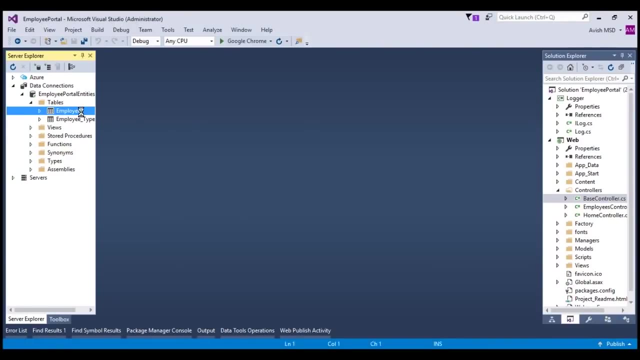 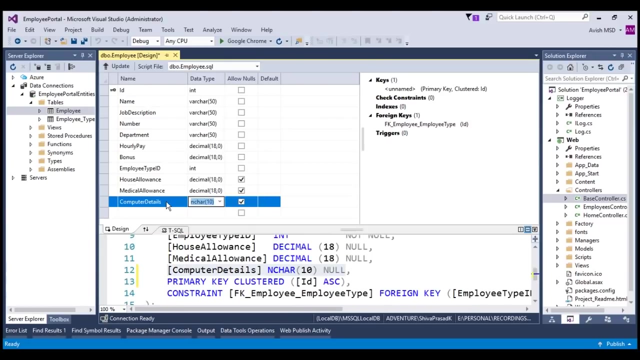 Dell desktops. The above business requirement can be achieved by leveraging on abstract factory pattern. Now let's bring up the visual studio and learn how we can implement the abstract factory pattern with our previous working example. Let's open the employee table and add a new column called computer details. Let's define the data. 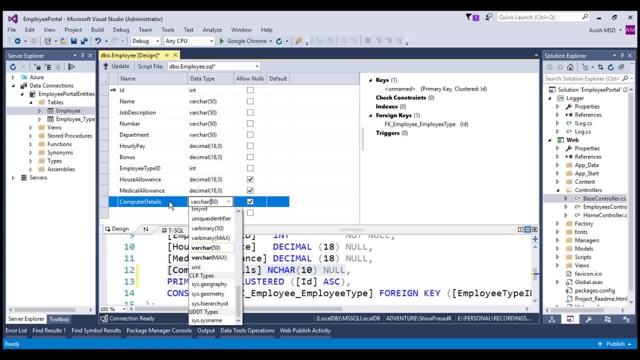 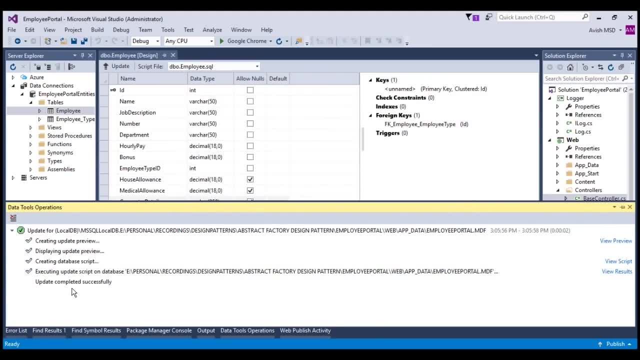 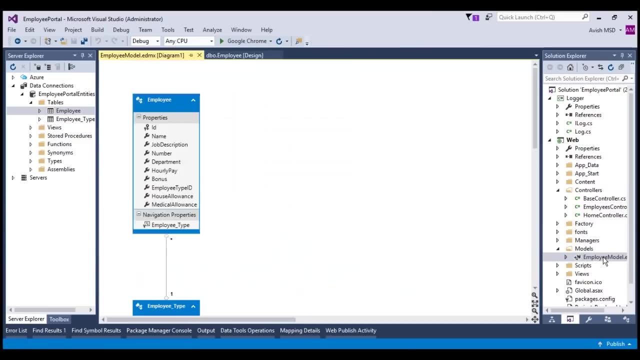 type as varchar. Let's make it as 250 and let's click on update. Let's click update database. Update completed successfully. Now let's switch to the models and open employee modeledmx and let's right click on this model and update model from the database. Let's click on refresh. 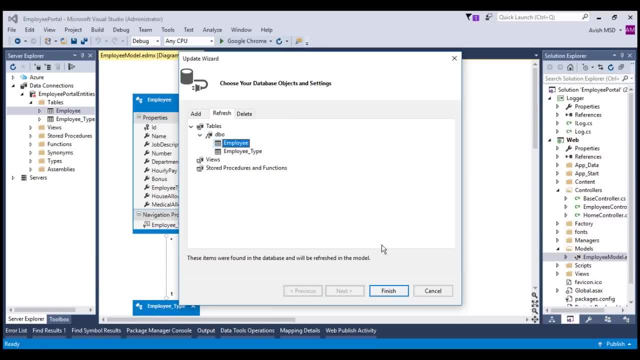 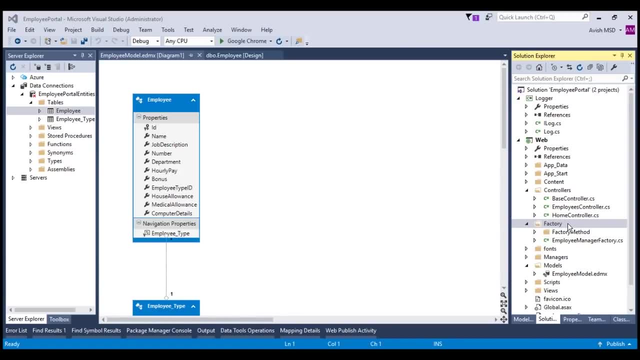 expand the tables and let's refresh the employee table. The changes are updated successfully. Now let's create a new folder under factory folder. Right click, add new folder and name this folder as abstract factory. Let's add some enumerations to support. 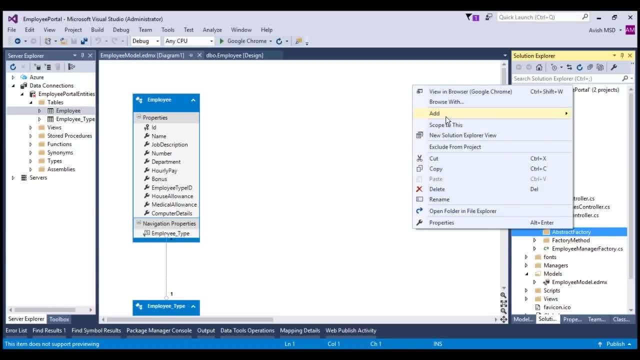 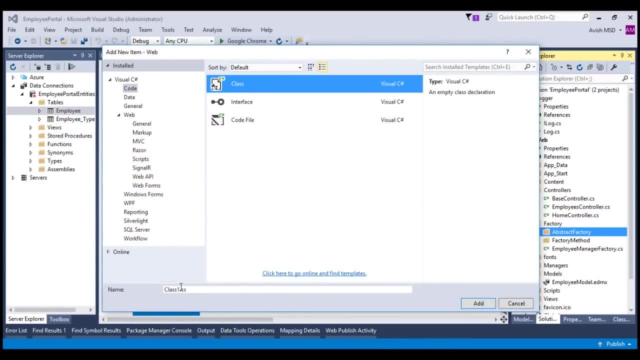 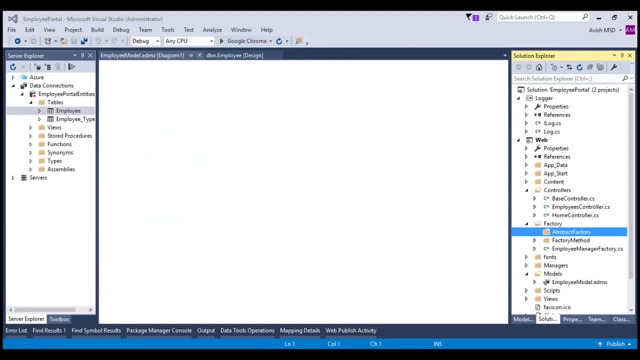 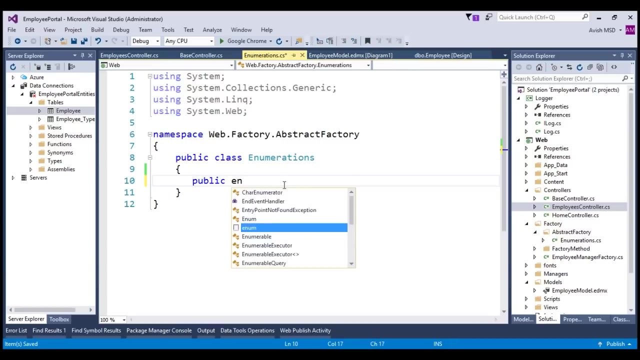 the business requirement. Let's right click and add new item and let's choose the class and name this class as enumerations. Let's create some new enumerations related to our business requirement. Let's first create public enum computer types, which are laptop and desktop. 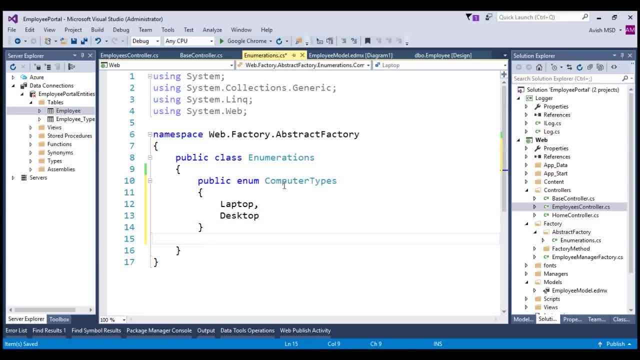 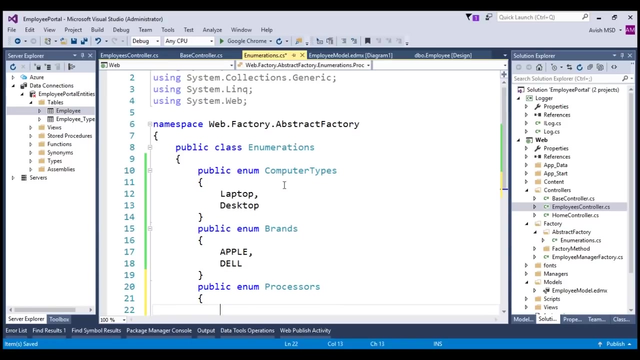 Let's create another enumeration and let's call this enumeration as brands, As we know that we need to hand out Apple and Dell brand desktops or laptops. Let's also create another enumeration and name it as processors, And let's create some processors as i3, i5 and i7.. 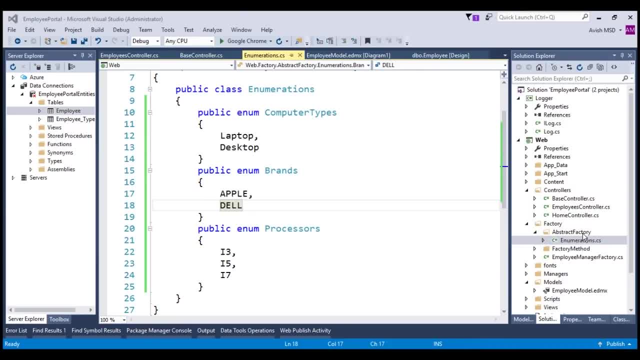 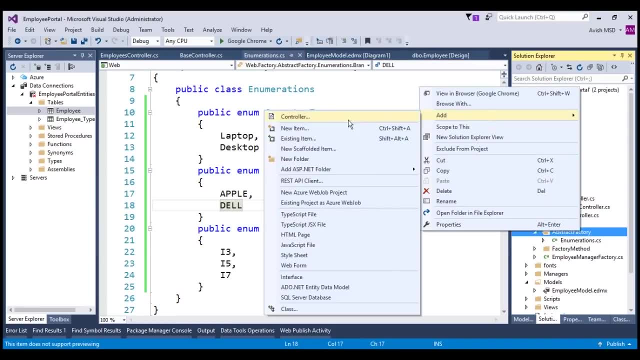 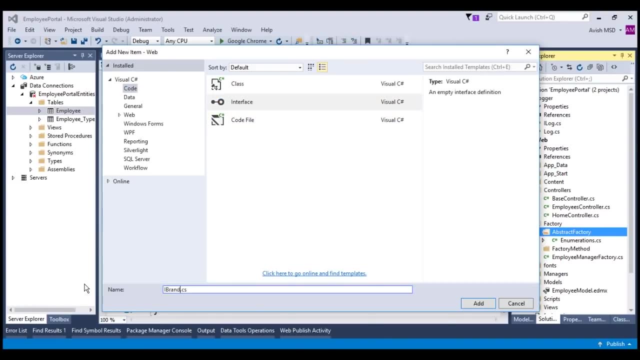 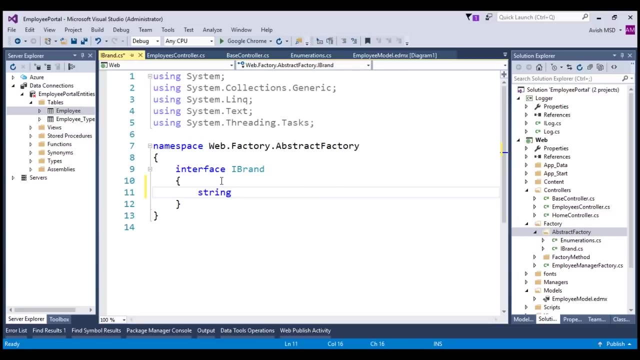 Let's now create abstract product interfaces. which declares a type of product. So I click on abstract factory folder- add new item. Let's create an interface and name this interface as ibrand, which returns brand name. So let's name this method name as get brand And the brand. 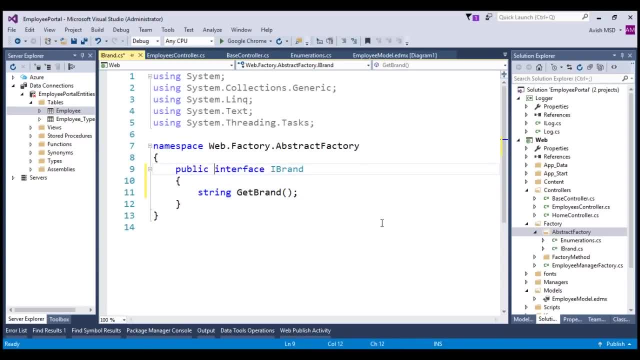 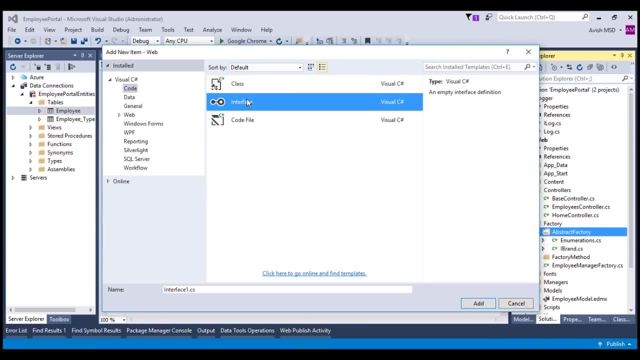 could be anything from ibrand to ibrand, So let's name this method name as get brand, Which could be Dell brand or Apple brand. Let's create another interface, add new item, choose interface and let's call this interface as i system type. 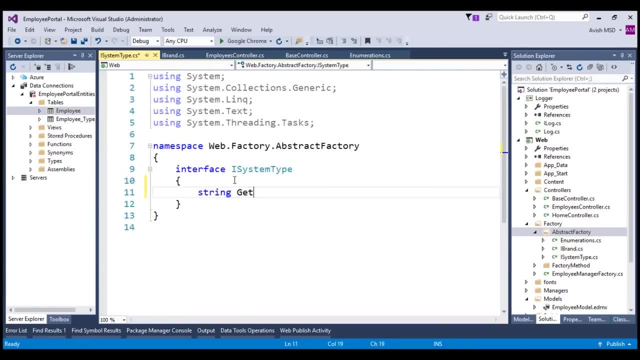 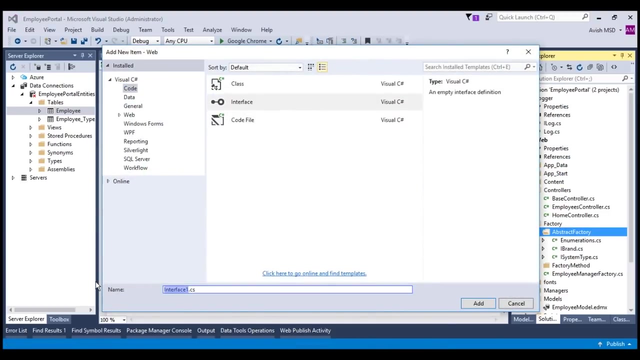 This interface will have a method which returns the system type and name it as get system type. Let's make this interface as public. Now let's create another interface named iProcessor. Right click, add new item, choose an interface and name this interface as iProcessor, which returns. 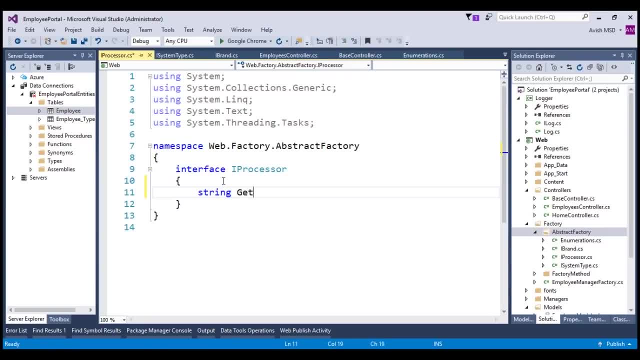 a processor, And let's create a method: get processor and make this interface as public. These three abstract product interfaces together compose a product which in our case would be a laptop or desktop with the specified configurations. Let's now implement these interfaces into concrete product classes. 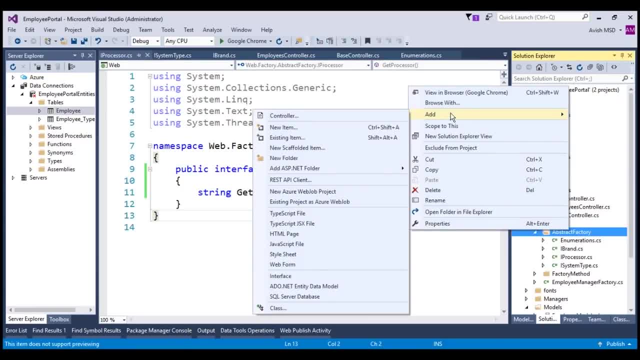 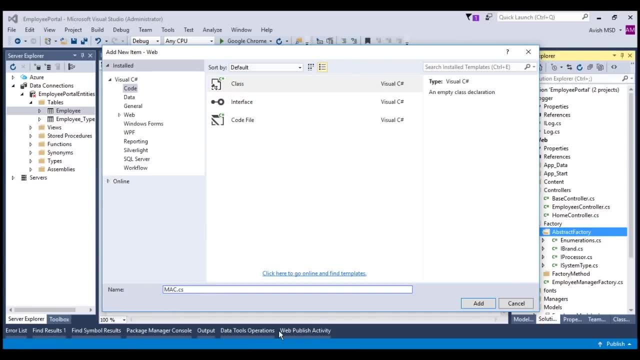 Let's right click on the abstract factory folder, add new item, choose a class and let's name this class as maccs. Let's name this class as maccs. Let's create a new interface for a Mac in which we can name: this one is: 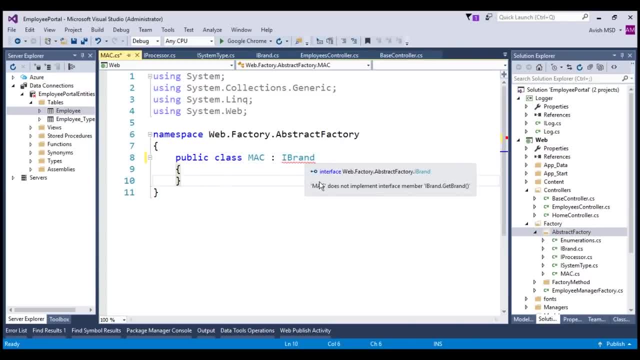 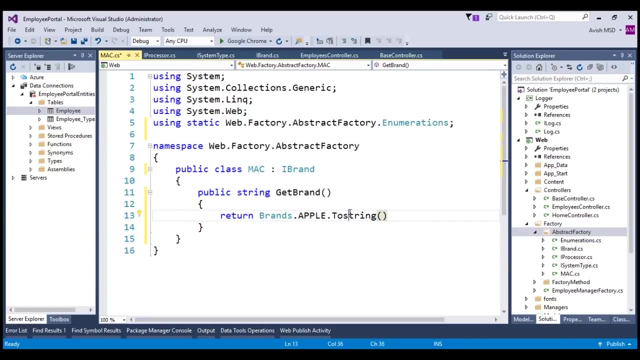 implements, Let's saybi-brand, which implements ibrand. Let's implement the ibrand method over here, which is getbrand, And let's return brandsappletoString. Let's resolve this issue by using the enumerations And let's return many more. 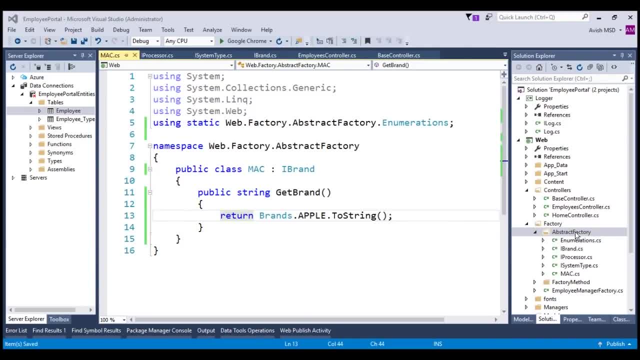 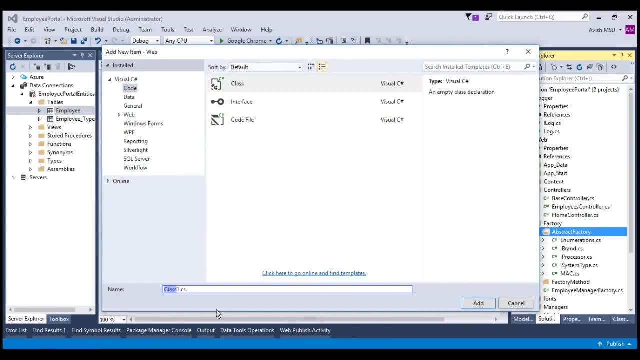 Let's remove this form- Let'sperson is the get brand- and let's create a new one for maccs and brandsappletoString. Let's create another class. Right click Add new item, Choose class and let's name this class as Dell, which implements the iBrand. 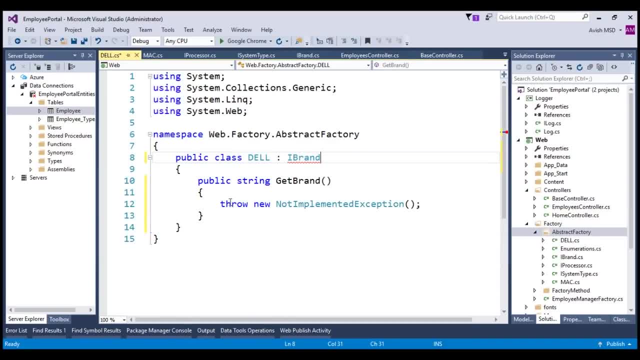 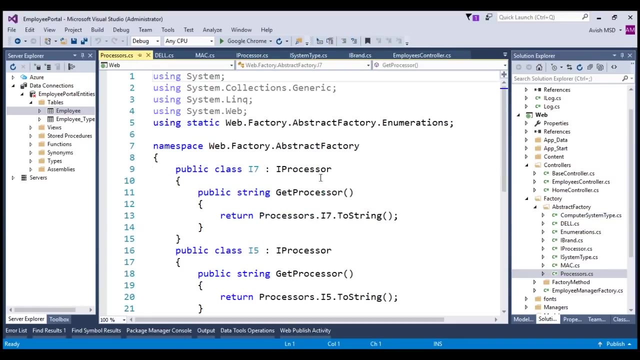 Let's implement the iBrand interface and let's return enumerations: brandsdelltoString. To save some time, I have already implemented the iProcessor interface for concrete products, which are i5 and i7.. I have also implemented the iSystemType to return the respective laptop or desktop as system types. Now that we have, 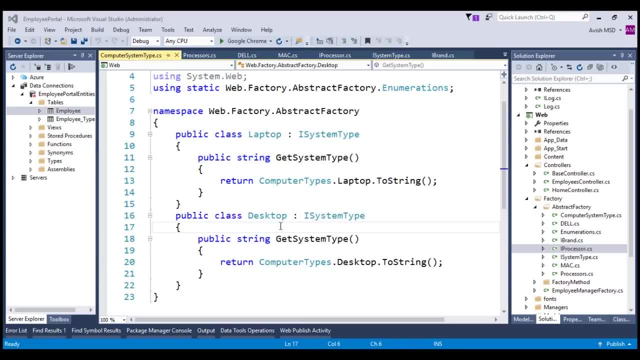 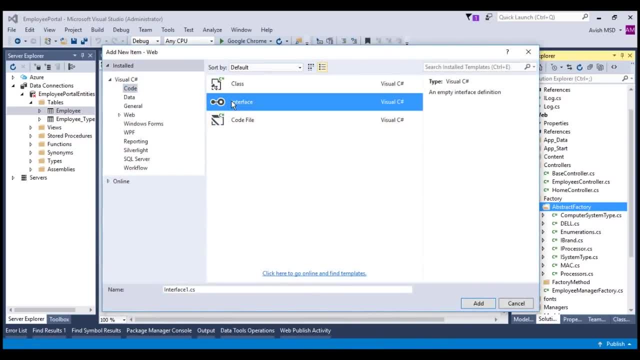 family systems. let's create a new system. Let's create a new system. Let's create a new system To create an interface of related products. let's create an interface which composes these products. Right click on abstract factory folder. Add new item. Choose an interface. Let's name this. 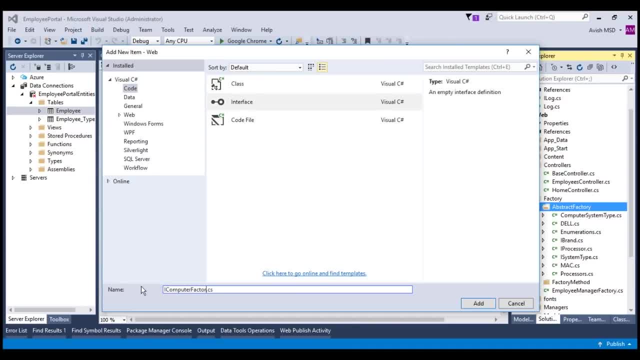 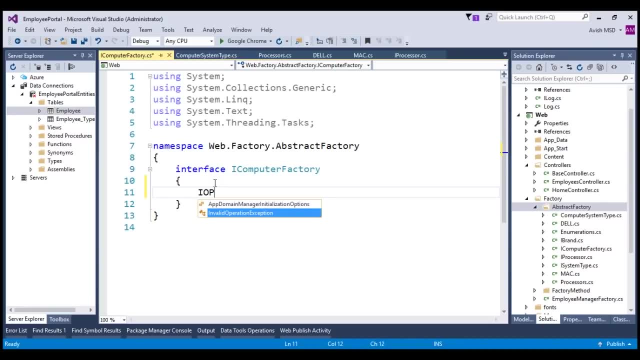 interface as iComputerFactory. Let's add the products that we have created to this interface, which are iProcessor- Let's name this as processor, iBrand Brand And iSystemType as SystemType. Now let's create concrete factories which implements this abstract factory interface. 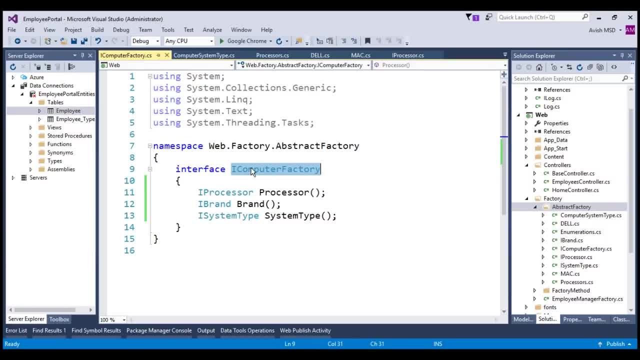 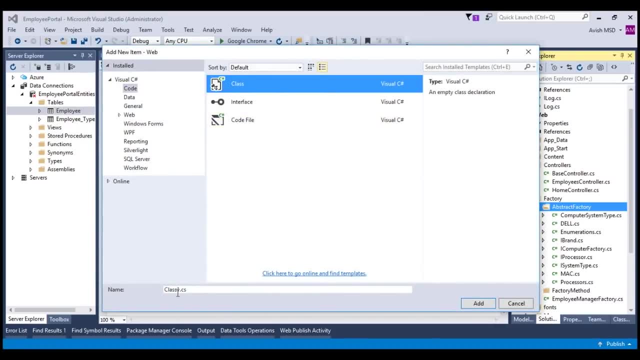 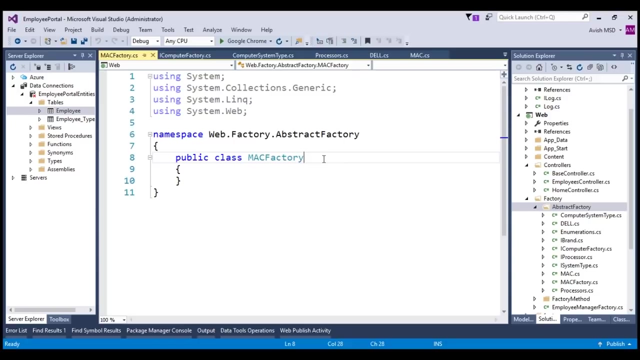 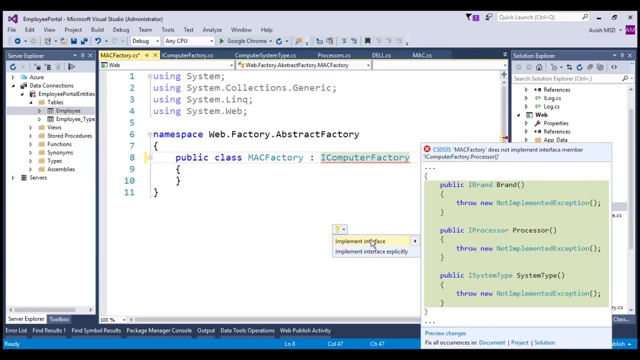 to create concrete products. Let's right click on this abstract factory folder, Add new item, Choose class And let's name this class as MacFactory so that it creates Apple laptop and desktop. Now let's inherit the iComputerFactory iComputerFactory And implement the interfaces. 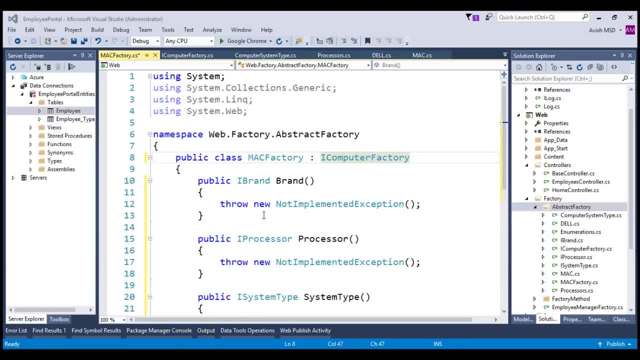 Now, when we need to create a MacFactory, let's say this is creating a new desktop, Then let's say i7, the brand would return as return new Mac, as the brand And the processor would be i7.. So let's say we will be creating a MacDos with i7, processor, i7 and the system. 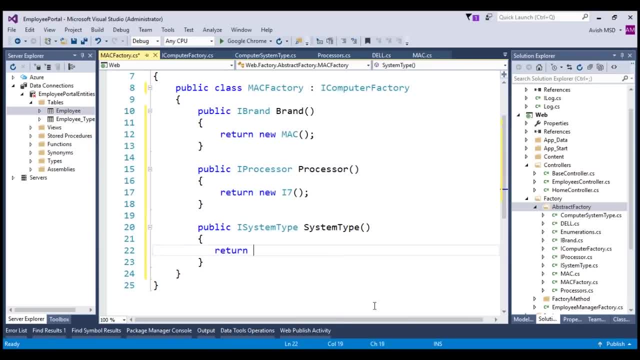 type would be: return new Mac. Now i7 would be i7.. Now i7 would be i7.. Now i7 would be i7.. Now i7 will be i7. Now i7 would be i7.. Now let's say we will create a MacDos with i7 processor. Let's say we will make 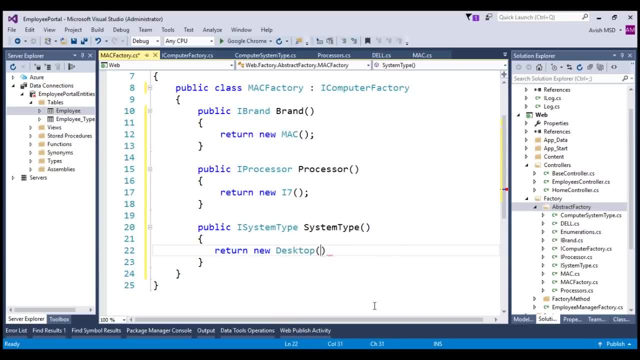 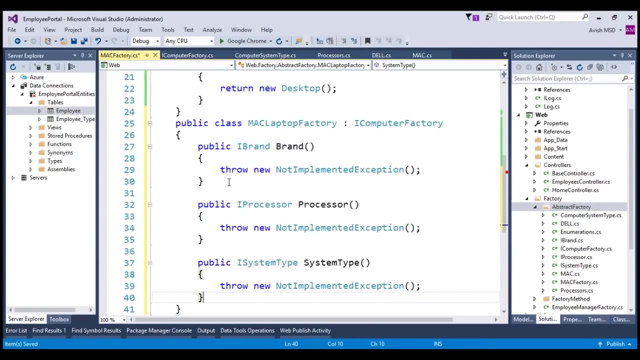 desktop. let's also create a Mac laptop factory. let's create it over here: public class Mac laptop factory which inherits iComputer factory. now let's implement the interfaces, implement interface and let's say the brand will be written new Mac and the processor will be written new i7 processor. 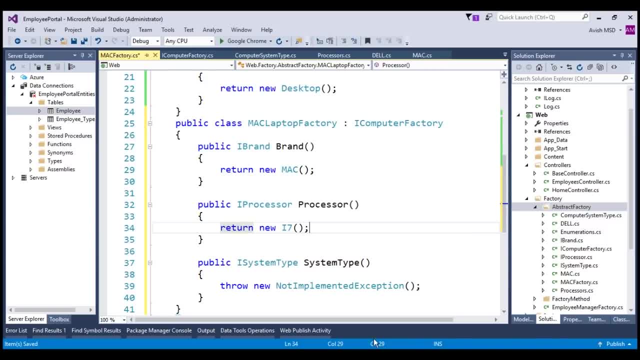 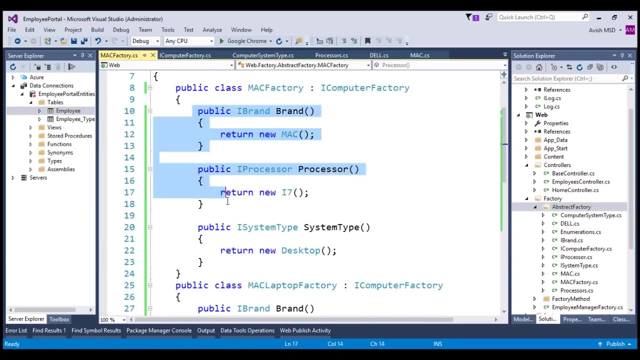 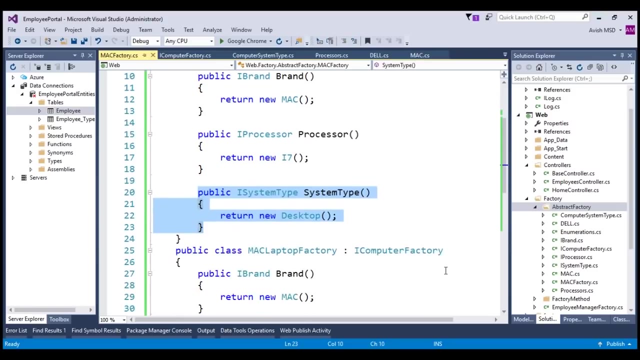 and the system type will be written. new laptop. and now, if you observe, the Mac factory and the Mac laptop factory- both has got the same brand, as well as the processor. the only difference between these two is the system type. so let's refine it further and, instead of inheriting the iComputer factory for Mac laptop factory, 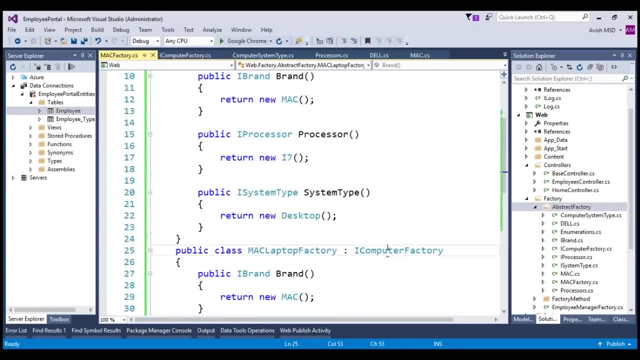 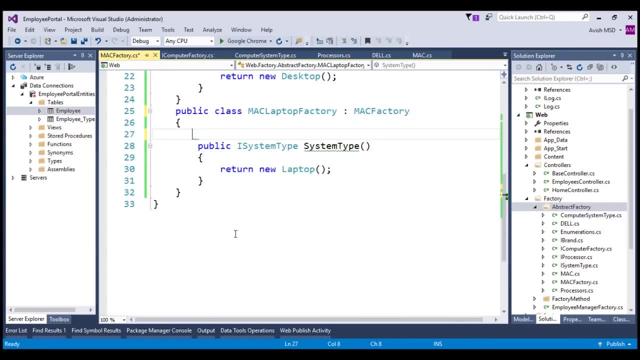 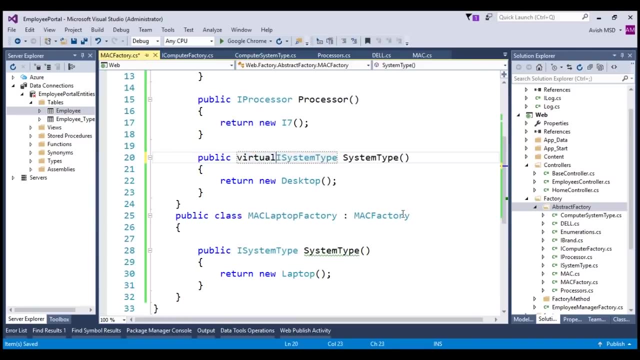 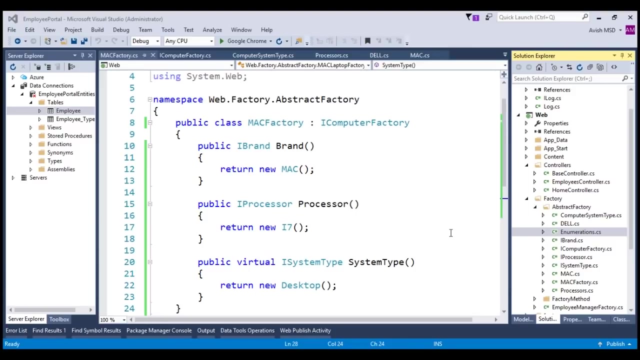 let's inherit from the Mac factory- say, Mac laptop factory inherits the Mac factory, and let's remove these implementations and change this implementation as virtual system type so that we can overwrite it here. let's now create concrete factories, which implements the abstract factory interface to create Dell products. let's right click on the abstract factory folder. 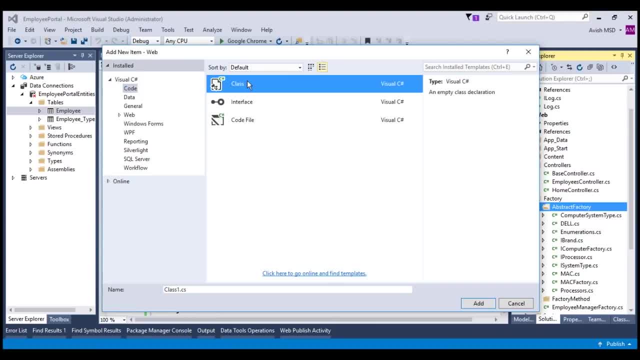 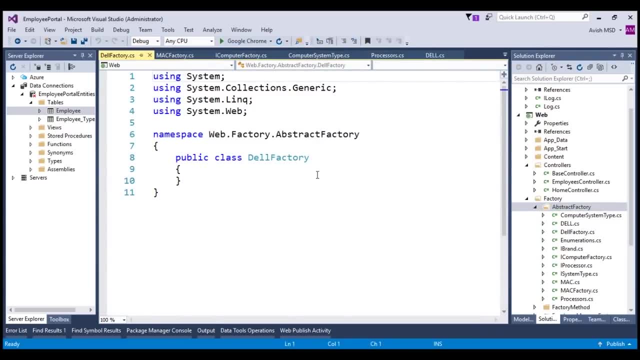 Add new item, choose class and name this class as Del factory, Which inherits from I computer factory. Let's implement the interface methods. implement interface and let's return. Return new del as a brand And let's return the processor as I 5. return new I 5. 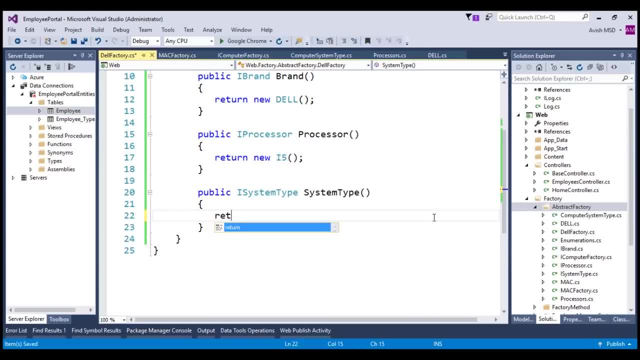 And let's return the system type as return: new desktop. Let's now create a laptop factory for del, similar to the Mac laptop factory. Let's say public class del laptop factory, Which inherits del factory, and We just need to overwrite the system type. So let's declare virtual. 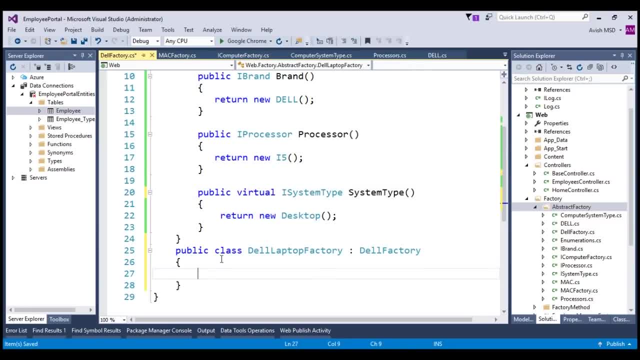 over here and Public over I High system type, Which is system type, and let's return new laptop. Now that we have implemented the abstract interfaces, as well as concrete implementations to those abstract interfaces and products, Let's see how we can address the business requirement. right click on the abstract factory add. 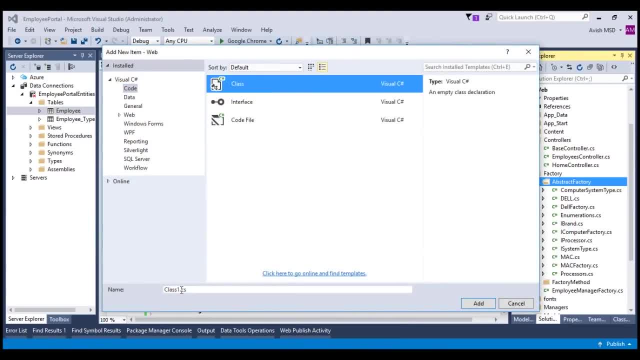 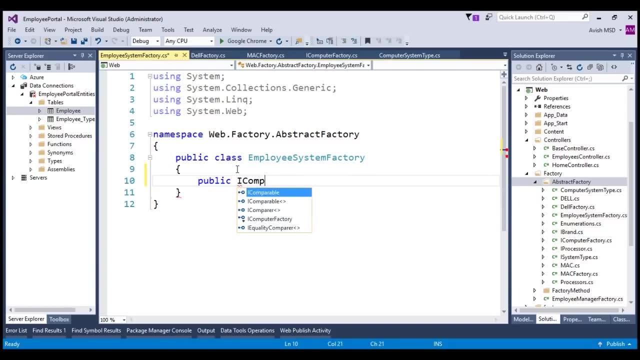 new item and choose a class and let's name this class as Employee system factory. Let's create a method, public, which returns I computer factory, And let's call this method as create, which adds: Accepts the employee as the input parameter. Let's resolve this issue By using web dot models. 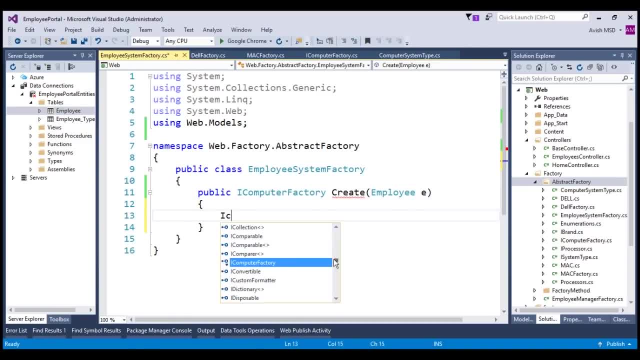 Let's declare the return value as I computer factory. I computer factory, return value equal to null. if e dot employee type ID equal to 1, which means he is a permanent employee, then if the employee's job description is manager, then for all the managers we are going to give laptop factories of apple, which means 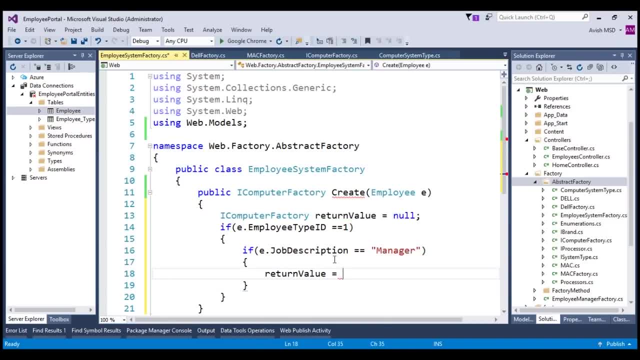 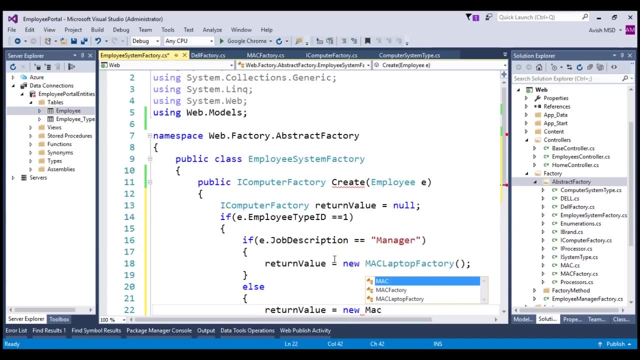 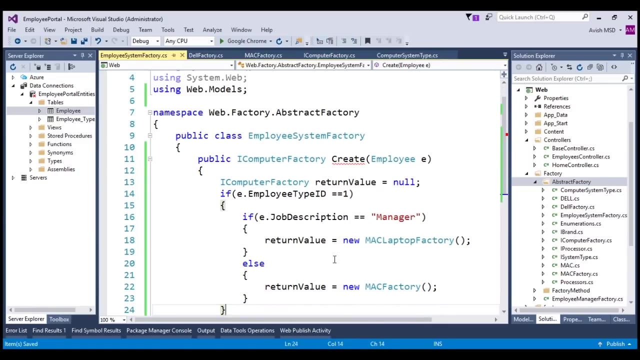 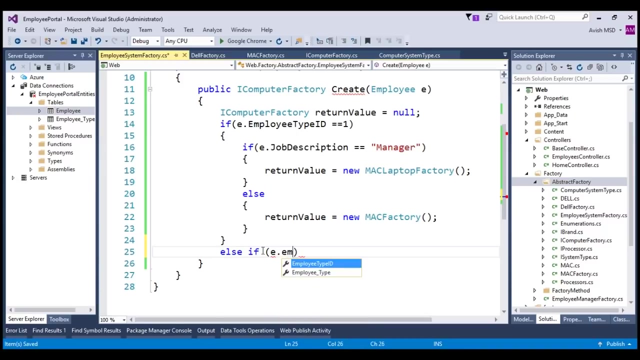 written value equal to new mac laptop factory other than managers. we are going to return or assign the written value equal to new mac factory. that means all the mac desktops. now, if he is a contract employee, which means else if e dot employee type id equal to 2. 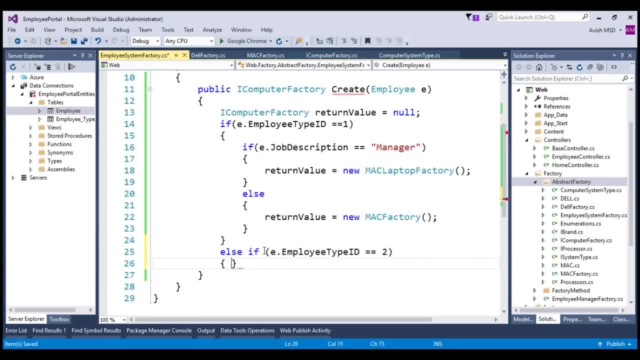 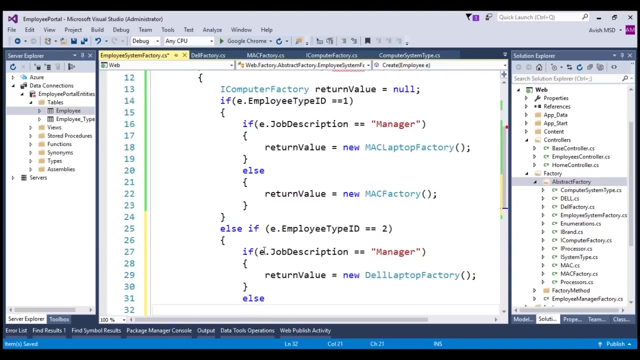 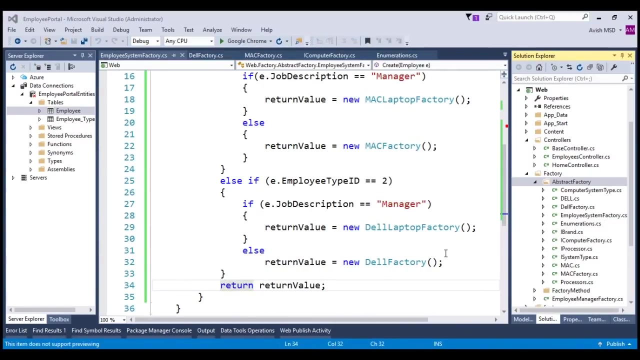 which means contract employee, employee. then if e dot job description equal to manager, we need to assign the written value as written value equal to new dell laptop factory, else written value equal to new dell factory. let's return the written value. return, return value. now let's create a client class which will be responsible to derive the system details. 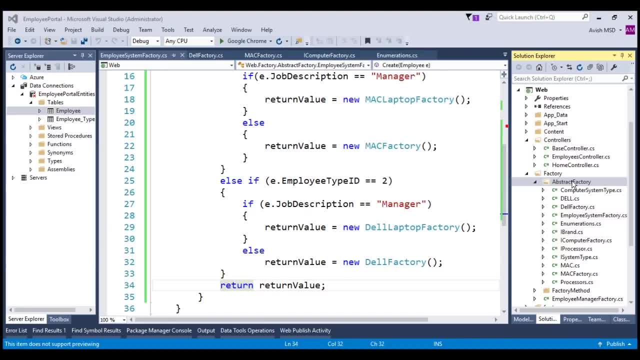 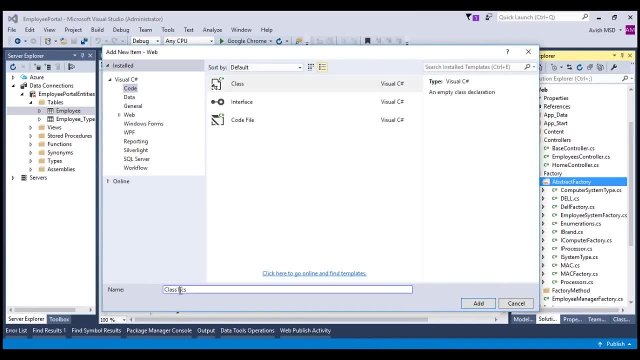 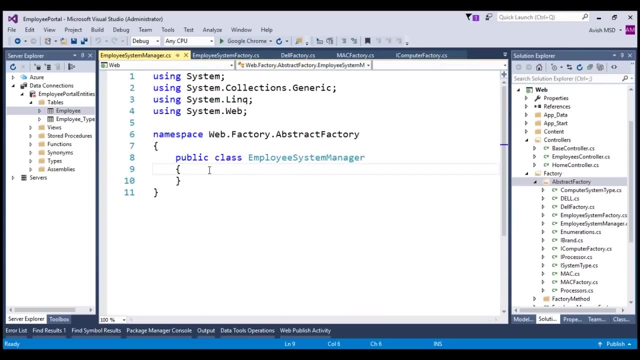 based on the created concrete factories. let's right click on the abstract factory folder, add new item, choose class and name this class as employee system manager. and let's create a icomputerfactory underscore icomputerfactory. let's create a constructor: public employee system manager. 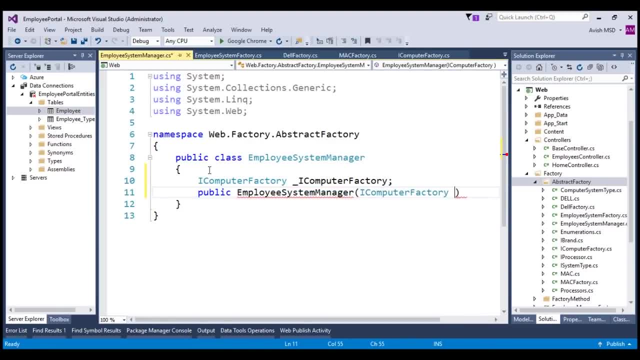 which accepts the input parameter as icomputerfactory- computer factory, and let's assign underscore: iComputerFactory is equal to iComputerFactory. Let's create a method- public String getSystemDetails- which uses this iComputerFactory and retrieves the respective brands, processor and system type- Let's say iBrand. 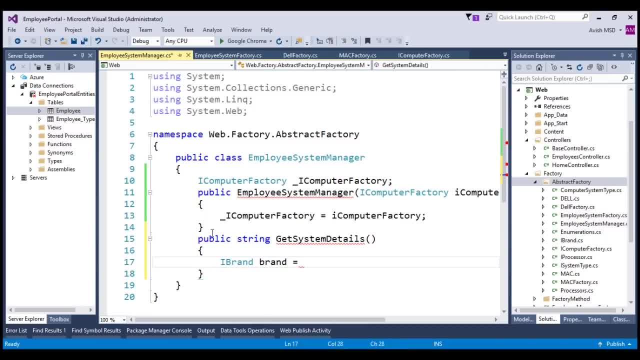 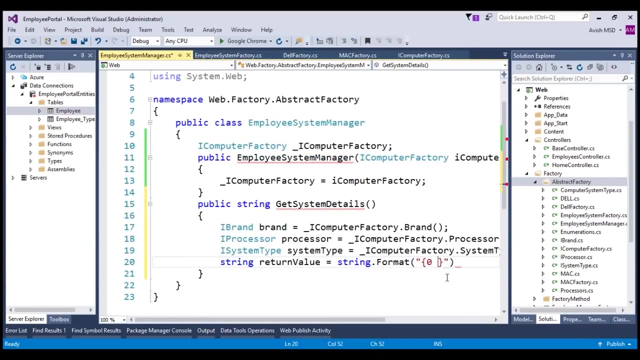 brand, equal to underscore iComputerFactorybrand. and. iProcessor: equal to underscore iComputerFactory. processor iSystemType. system type: equal to underscore iComputerFactory system type. Let's assign the return value as String. return value equal to StringFormat of 0 and 2. 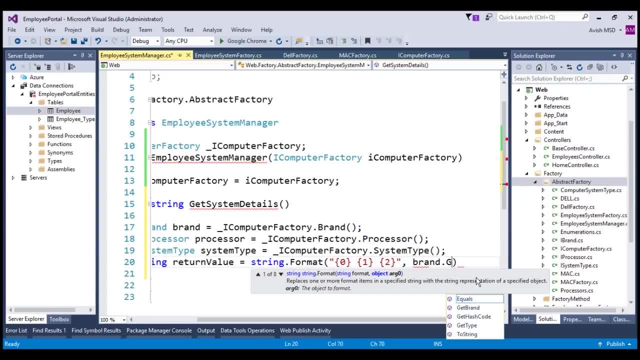 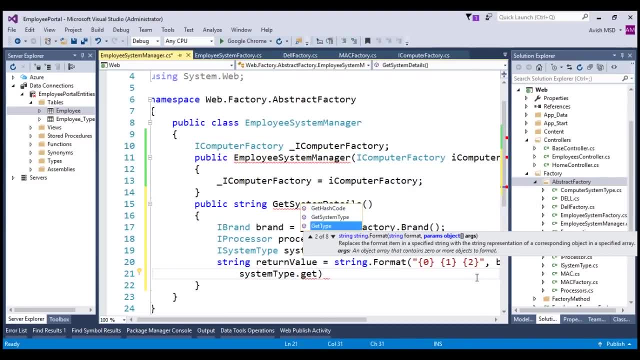 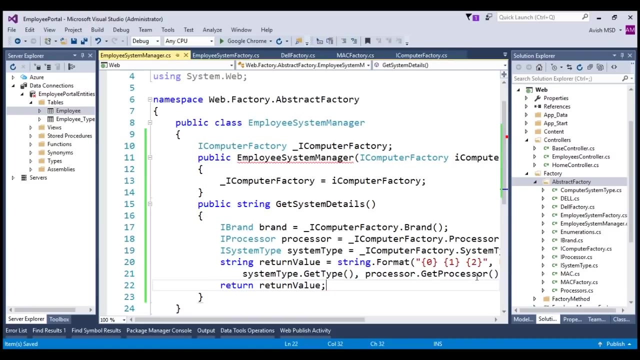 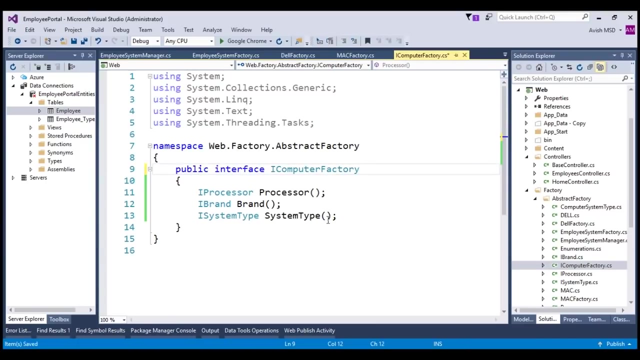 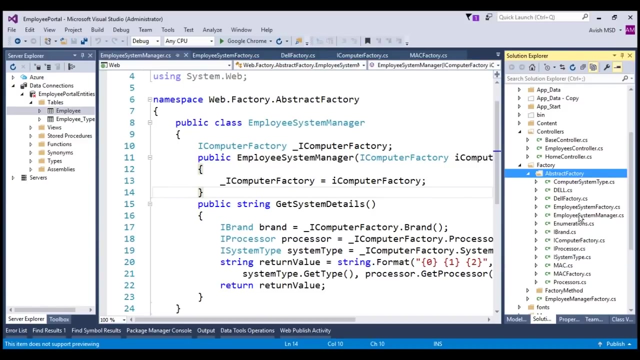 which means brand- getBrand, comma, systemType dot- getType, and processor- dot- getProcessor. return- returnValue. Let's resolve this error by making the sci-computer factory, as a public interface, public, and let's switch back. Let's rearrange all the classes under the abstract factory folder, based on the. 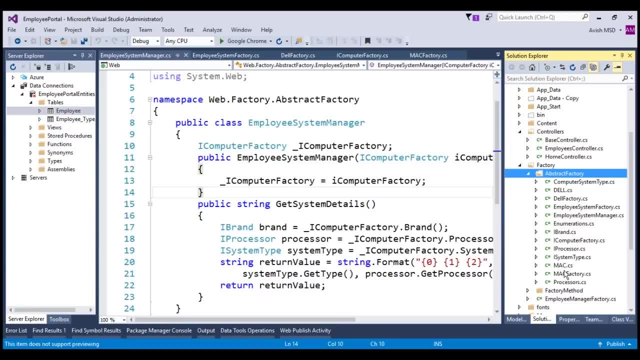 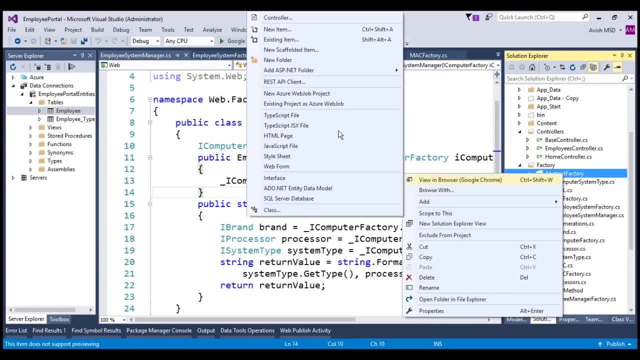 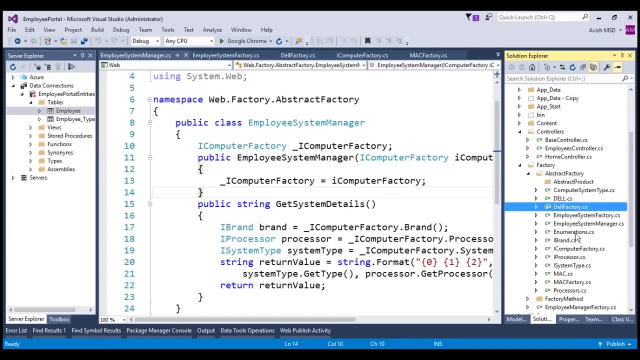 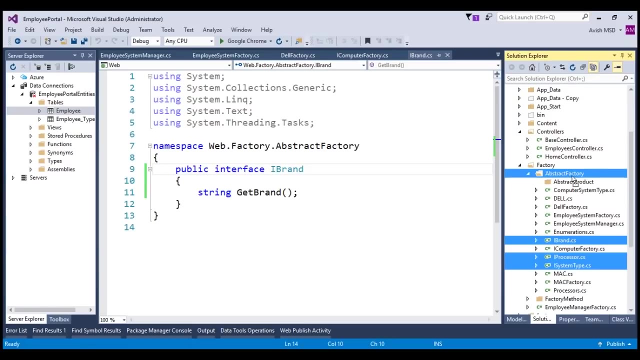 representation diagram which we have illustrated in the starting of this tutorial. Let's create a folder- abstract product- right-click, add new folder and name it as abstract product, and let's move iBrand- iProcessor- iSystemType under the new folder. Let's create a folder called. 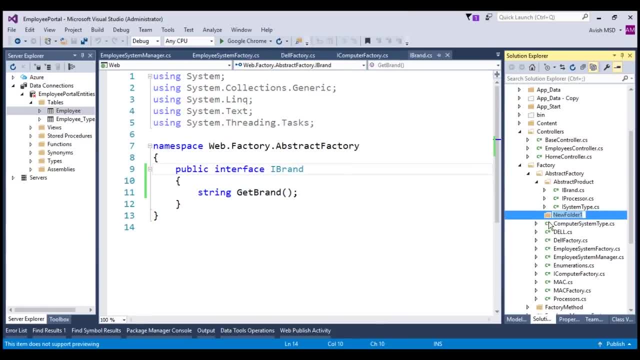 concrete product: right-click, add new folder and say concrete product and move all the concrete product implementations under this folder, which are Mac, Dell processors and computer systems. Let's create another folder, add new folder and name this folder as concrete factory and let's move implementations related to. 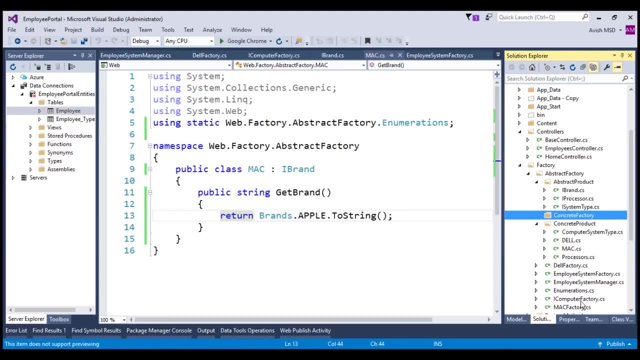 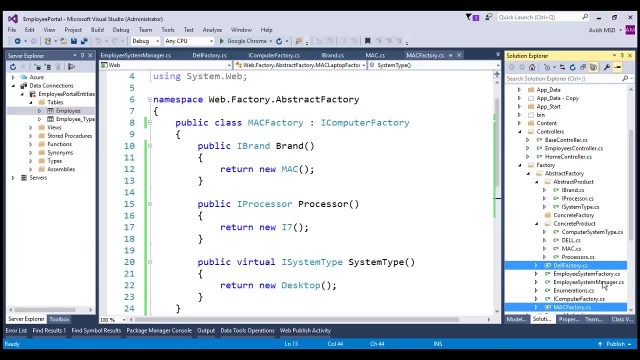 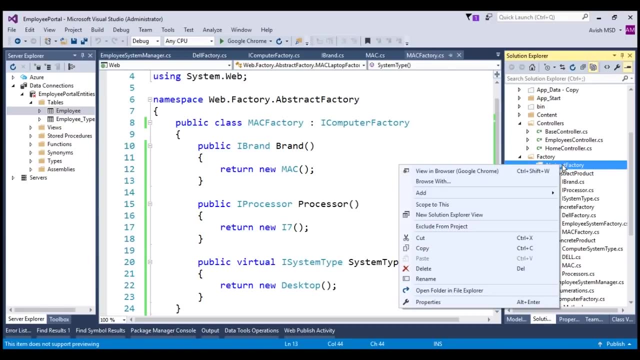 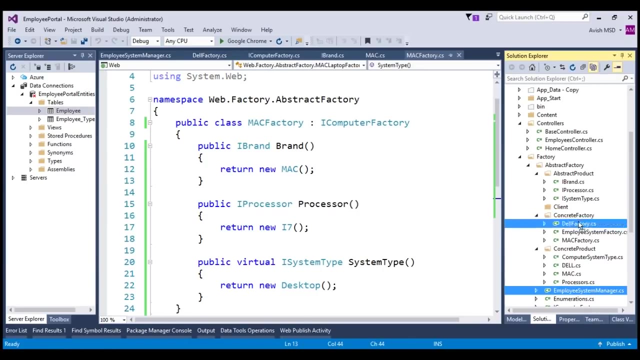 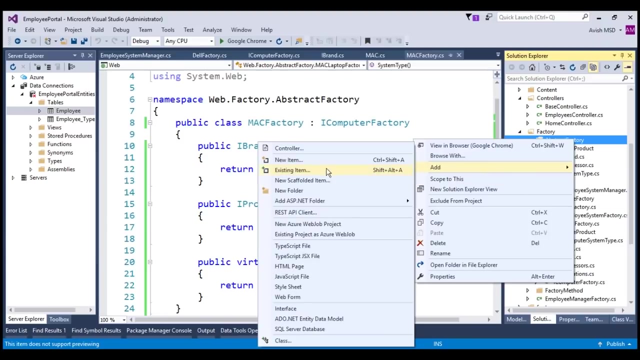 abstract factory interface. So let's move Mac factory, Dell factory and employee system factory into this folder. Let's create another folder and name this as client- new folder: client- and let's move the employee system manager under this folder. Let's also create a folder named abstract. 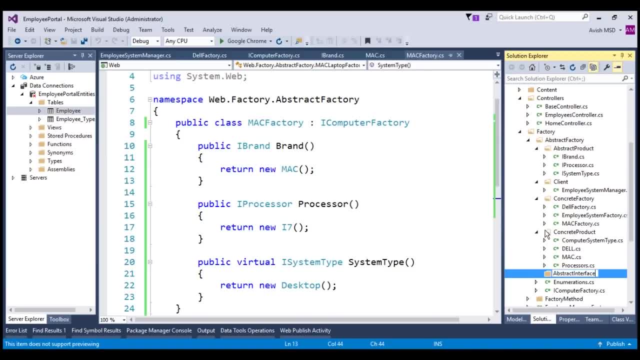 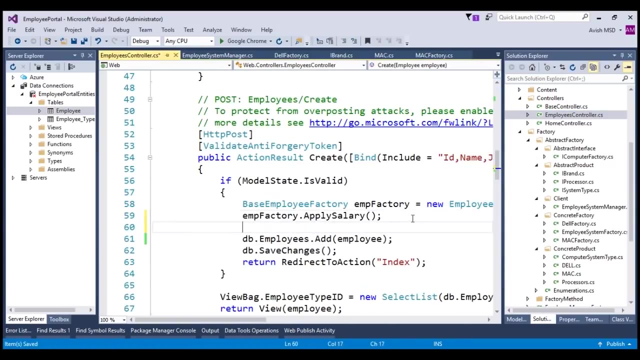 interface and let's move iComputer factory and any that. I hope now you are clear with what we have implemented till here. Let's now integrate these changes and implement the requirement in the employees controller. Let's open the employees controller. Let's create the abstract factory here: iComputer factory. 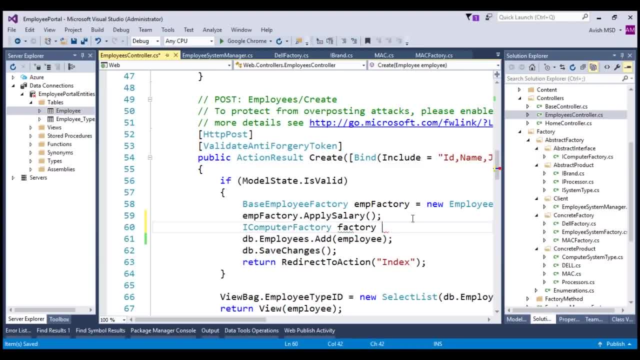 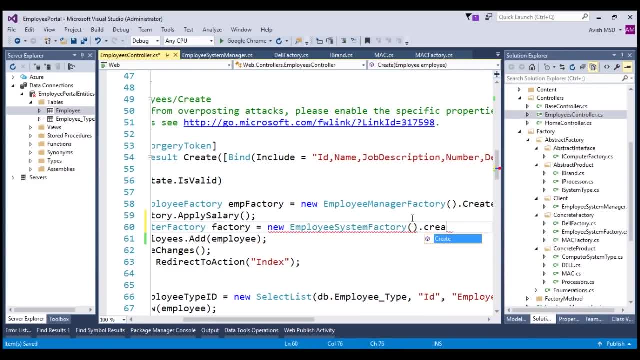 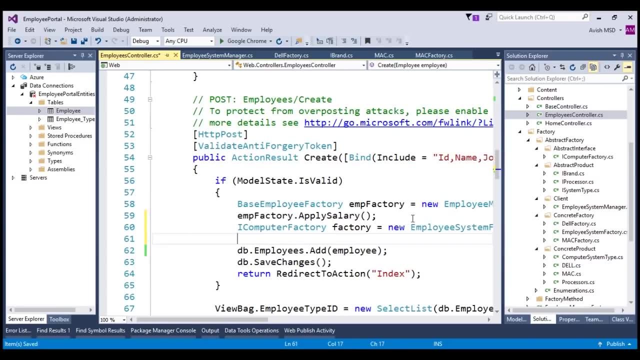 factory Factories- yours, go to new employees system, factory 木- and let's pass the employee as an input parameter for the create method. Now let's use the client which we have created, which is Effective, sustain of employee manager based starting client and which isn't ran capture project v1. let's run this method to execute an. appropriate core. Next, I am going to than clickуб. I am justvergin reply. so if I do, are I'm going to send this file to Microsoft practicum? Leave me alone die, or have a amount of money for this file and access any of this logic network command들을. Leave me alone die if I have no other. Robin Power. author. New Employees وأ� propek Щ вы Geneva кadiananya insurance manager i4 as well. 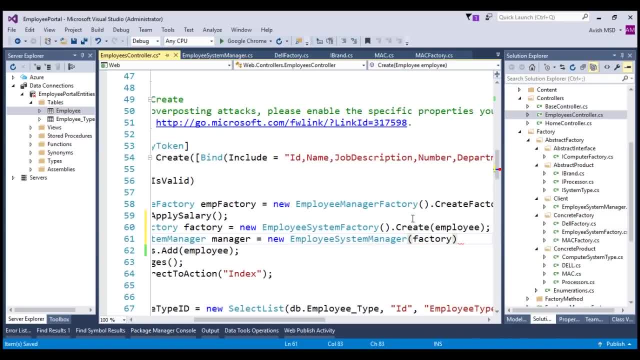 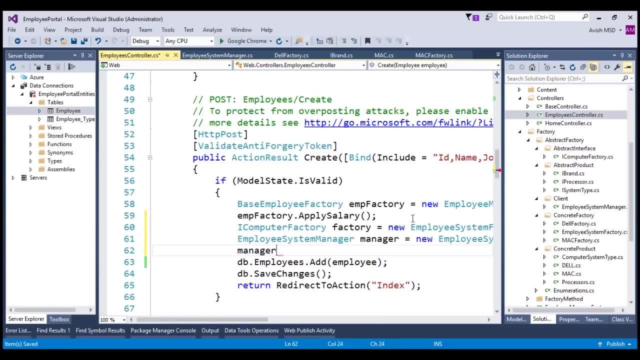 and let's use a client which we have created, which is employee system manager managementarm revenue. this is on Contra of a new employee system manager and which I accept. this abstract factory, as in EPSMoso, walls basically ul9 factory manager dot. get system details, will retrieve the respective systems. 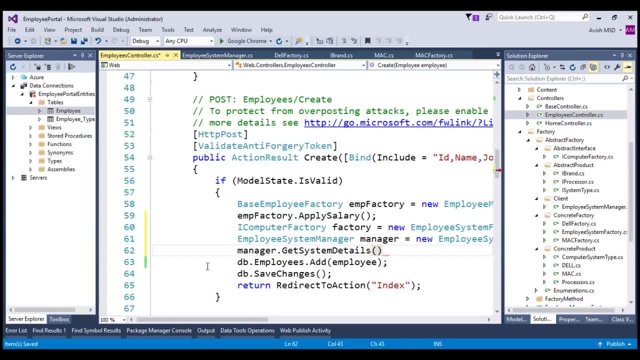 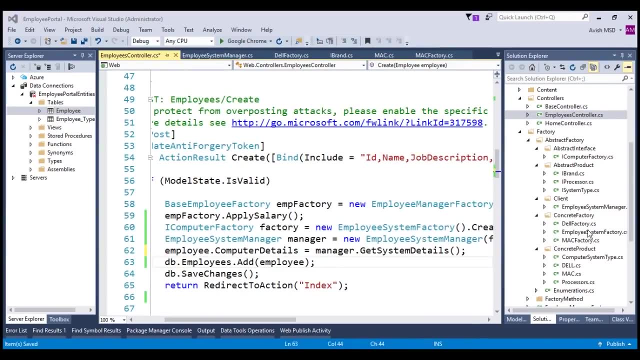 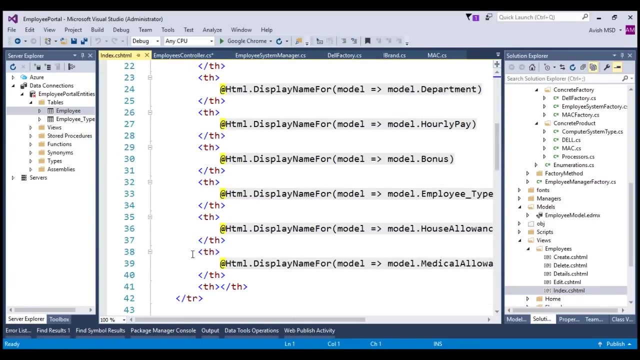 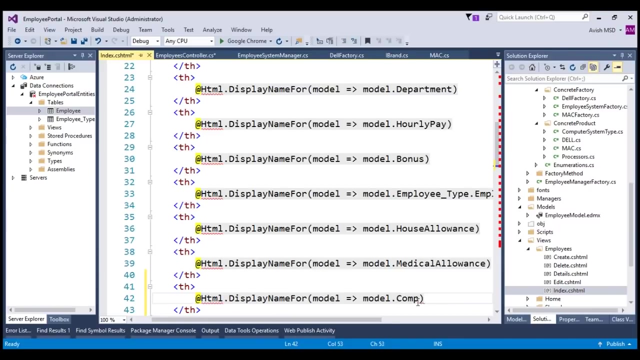 that we are handing off to the employees. so let's say: employee dot computer details equal to manager dot get system details. let's now switch to the views: expand employees and let's go to the index view and let's add this new column that we have created in the header, which is model dot computer details. 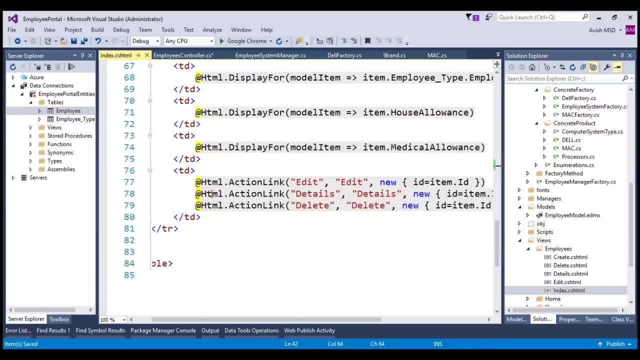 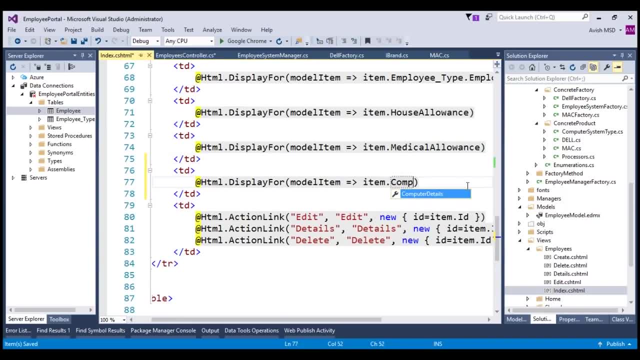 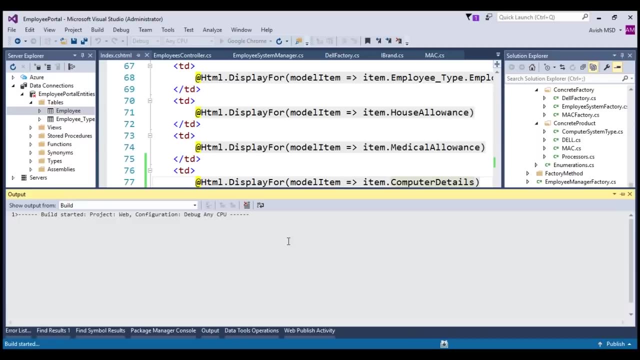 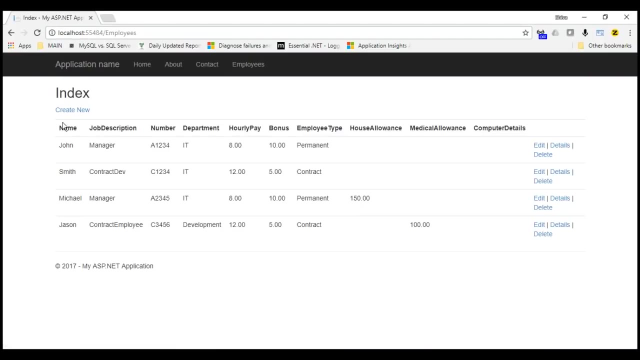 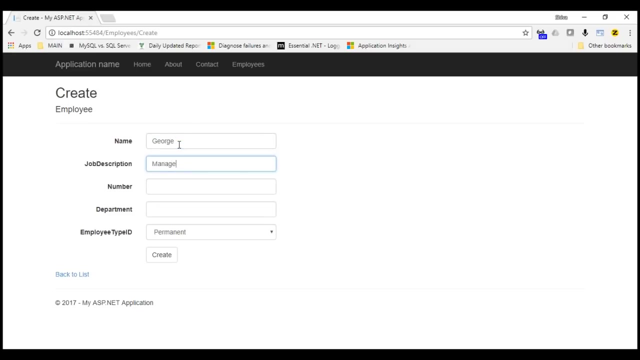 let's also add this in the table data. let's use the existing one and change this to computer details. let's compile this application and let's run this application. let's click on employees and create a new employee. the name as George, Job Description as Manager, P3456 as the number and Department as IT. 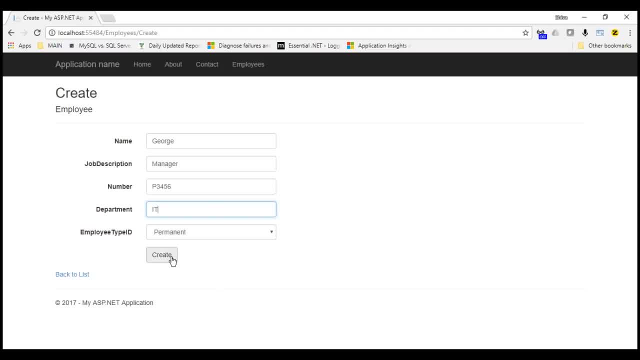 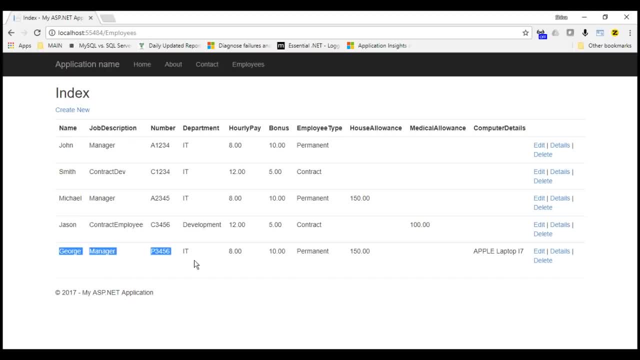 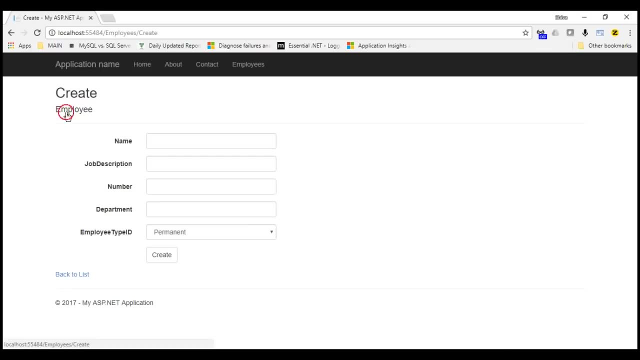 Let's choose the Employee Type ID as Permanent and let's click Create. Notice that George, who is a Permanent Employee and a Manager, is allotted an Apple Laptop i7.. Let's create another Employee and let's name the new Employee as Sebastian and let's put 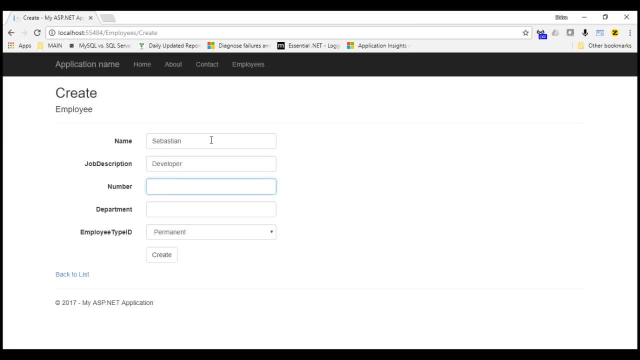 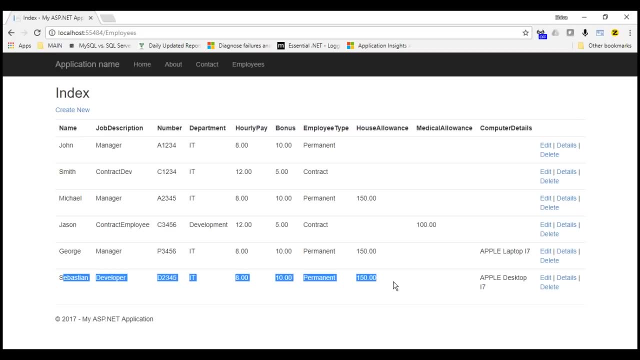 the Job Description as Developer and the number as D2345,. Department as IT, and let's choose Employee Type as Permanent here as well. Let's click on Create. Look at that Sebastian is created as Developer with a Computer Details ID. Let's name this Employee as Apple Desktop i7.. 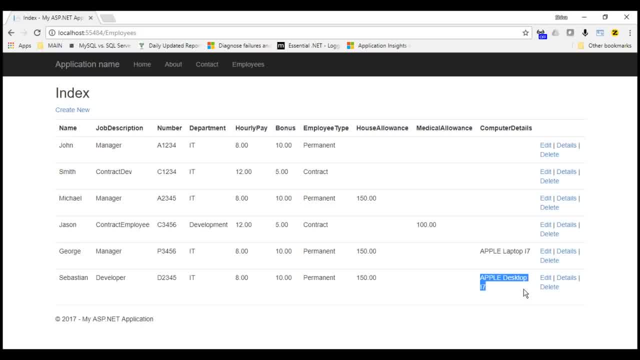 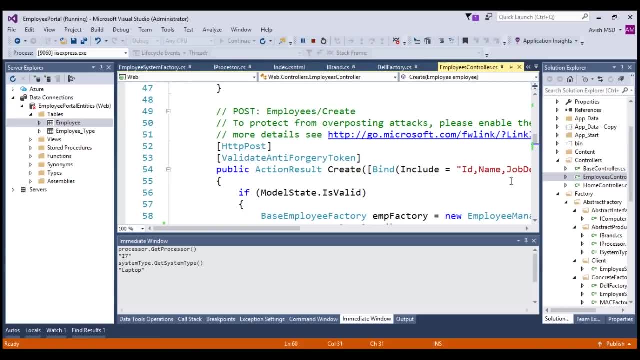 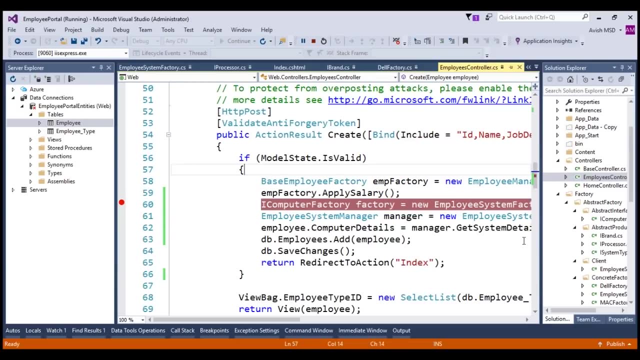 Now, before creating a Temporary Employee, let's try to debug this application and see how it behaves. Let's put a breakpoint over here at the Create method, and let's run through this application. Let's create a new Employee. Let's name this Employee as Andrew. 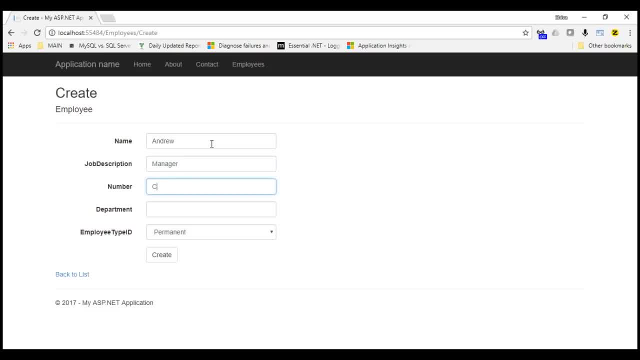 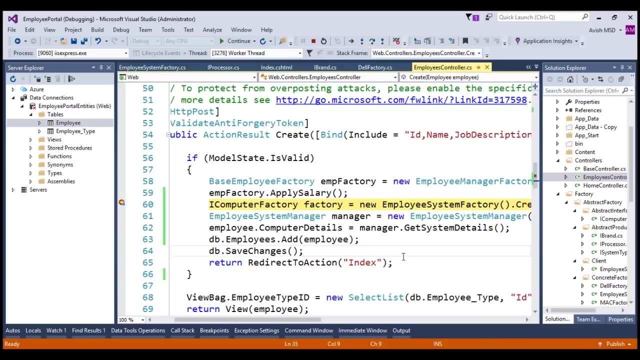 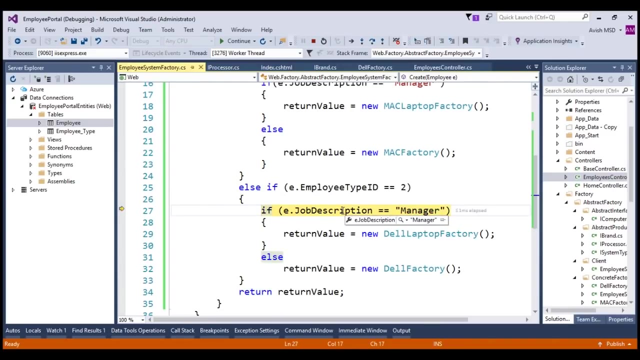 Job Description as Manager, Number as C3456.. Department as IT. and let's change the Employee Type to Contract. Let's click on Create Now let's step into this code. Notice that, since the Employee Type ID is equal to true and the Job Description is Manager, 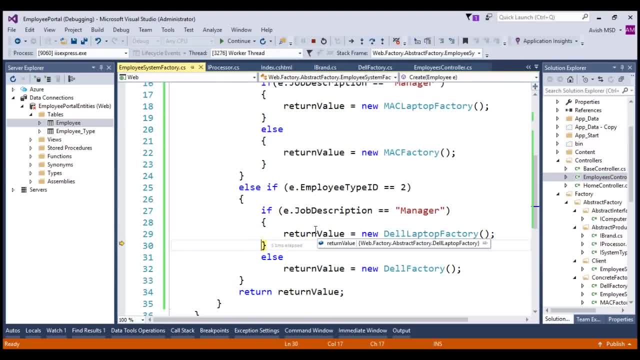 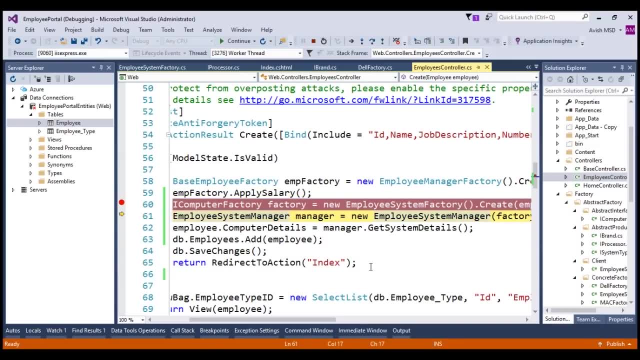 we are creating a Dell Laptop Factory And we are returning the AppStack Factory back to the Client. Let's step in through the Client. Look at that. The AppStack Factory is getting initialized over here, And then we are invoking the Get System Details, which invokes the respective Brand Processor. 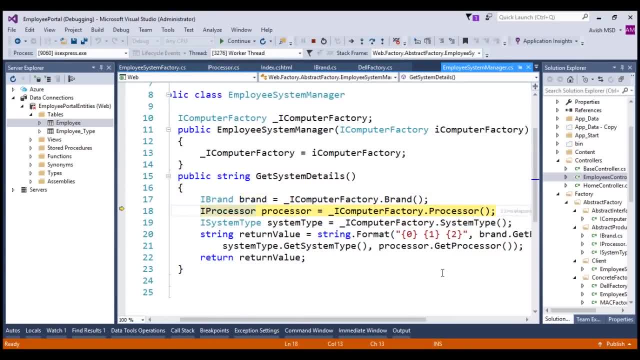 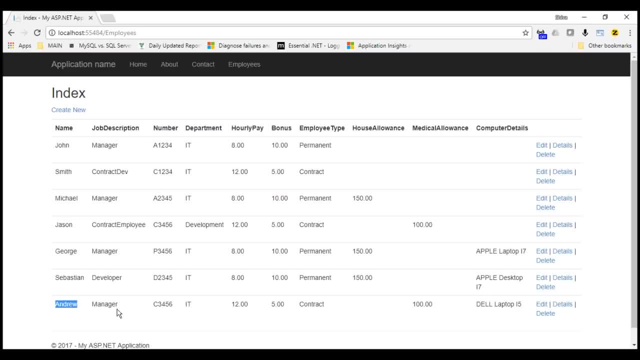 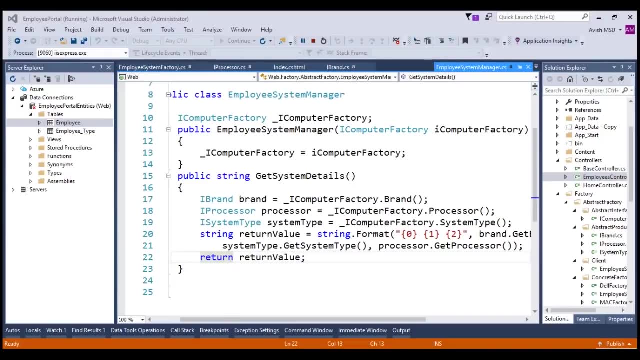 and System Type and retrieves the corresponding values. Let's press F5.. Now notice that Andrew, who is a Contract Manager, is allotted with Dell Laptop with I-5 configuration. With this, we have successfully addressed the requirement by using the AppStack Factory. 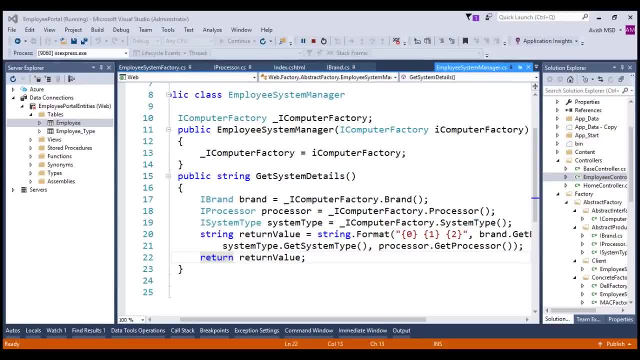 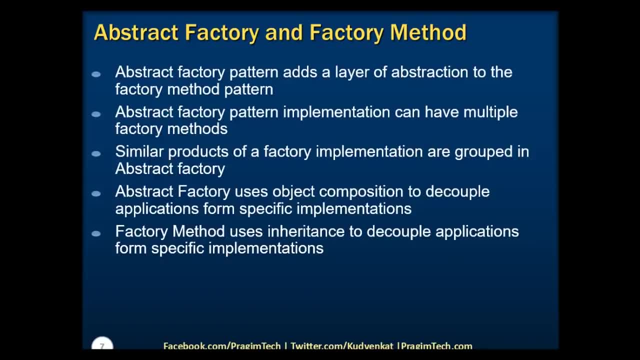 Design Pattern. Now let's take a look at the major differences between AppStack Factory and Factory Method Pattern. The AppStack Factory Design Pattern adds a layer of abstraction to the Factory Method Pattern. The AppStack Factory Pattern Implementation can have multiple Factory Methods.